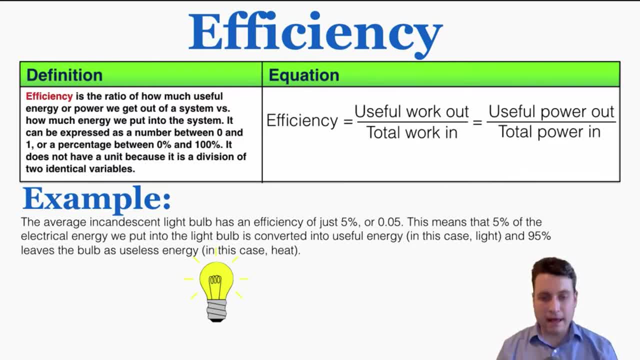 the situation. as an example, the average incandescent light bulb has an efficiency of just 5% or 0.05.. This means that 5% of the electrical energy we put into the light bulb is converted into useful energy. And because this is a light bulb, when we use it we usually want. 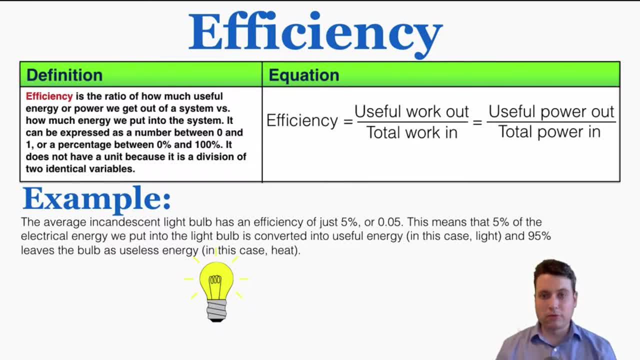 to get light out of it. So we consider the useful energy to be whatever radiant energy or light energy we get out of this machine. If it's just 5% efficient, that means that 5% of the electrical energy that goes in gets turned into radiant energy, the stuff that we want. And if it's 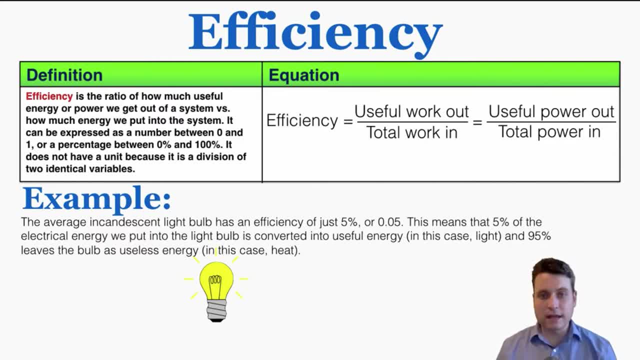 5% efficient, then 95% leaves the bulb as useless energy. In this case it leaves it as heat. specifically, Whenever we use an incandescent light bulb, no matter how much electricity we're putting into it, only 5% comes back to us as useful radiant energy and the rest is lost as heat to the 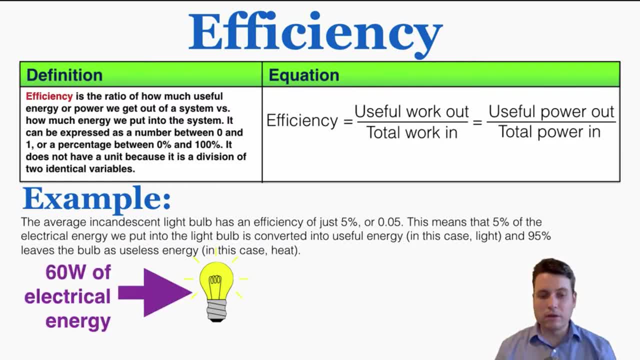 environment. As an example, if an incandescent bulb is a 60 watt bulb, that means that 60 watts of electrical energy are going into the bulb but only 3 watts of useful radiant energy- just 5% of that 60, are coming out of the bulb as radiant energy. and the rest, the other 57 watts, 95% of. 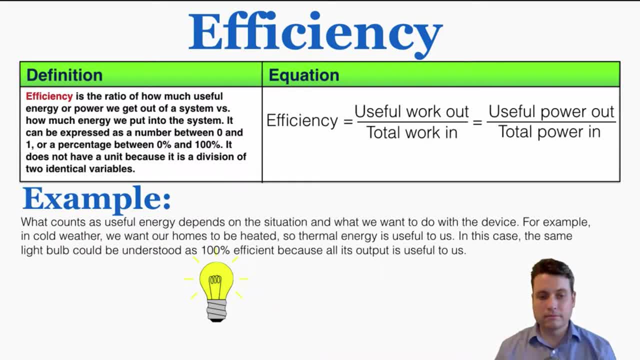 the energy are going into the bulb. So if we're looking at a light bulb and we're looking at is coming out as useless thermal energy, And again what counts as useful energy really depends on the situation and what we want to do with the device. For example, in cold weather, we do want. 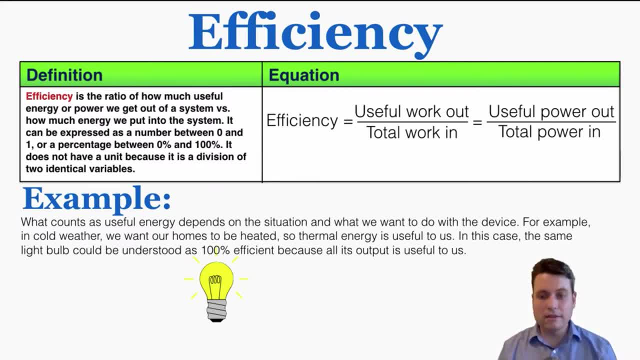 our homes to be heated. so thermal energy is useful to us, And in this case we could possibly say that the light bulb could be understood as 100% efficient, because all of the energy is useful and valuable to us. So what counts as useful energy is kind of subjective and based on the problem. 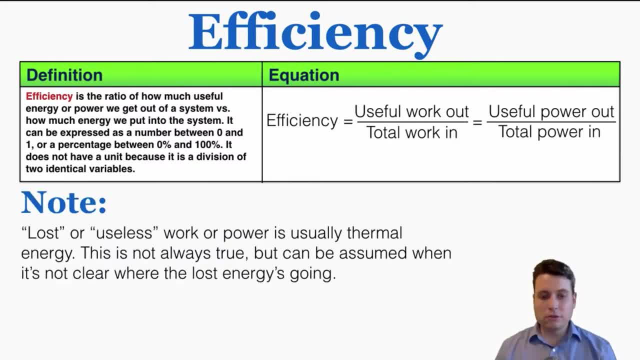 that you're trying to solve with the machine. Just as a note, lost or useless power or work is usually used to solve problems. So if we're looking at a light bulb and we're looking at thermal energy, when we talk about that we usually mean heat leaving a system. This is not. 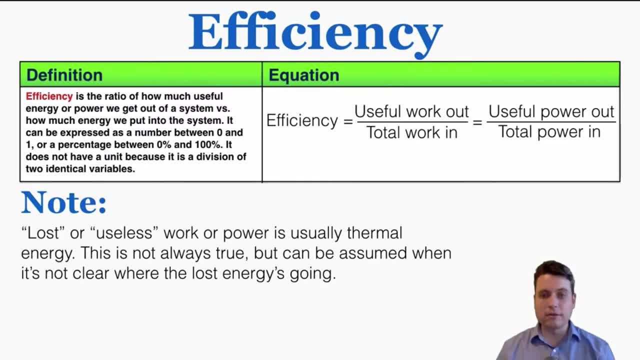 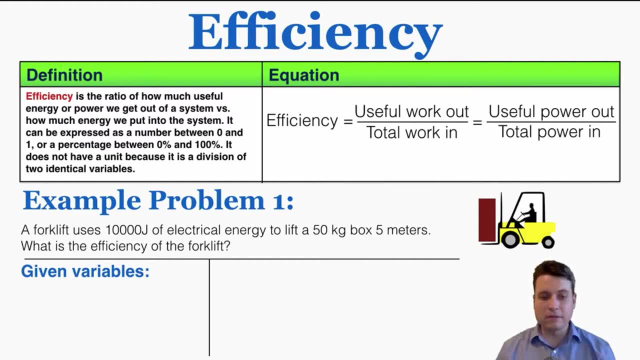 always true, but it can be assumed when it's not clear where the energy is going. Here are a few example problems. In this first one, a forklift uses 10,000 joules of electrical energy to lift a 50 kilogram box 5 meters. What is the efficiency of the forklift? We know that the total work in 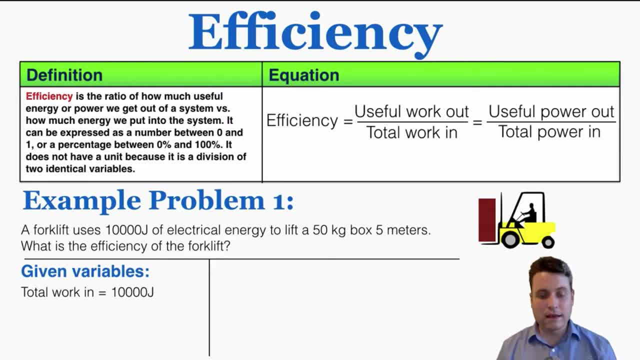 is equal to 10,000 joules of electrical energy. It's using 10,000 joules of energy to perform this task And I can see that the change in potential energy as it lifts the box is going to be from 0 to. 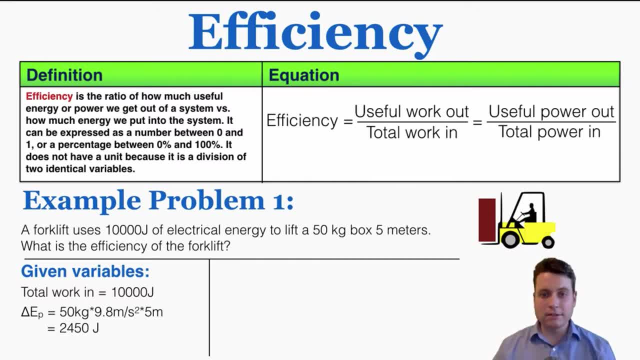 5 meters. So if we're looking at a light bulb and we're looking at a light bulb and we're looking at a box, 5 meters, so the change is just going to be the potential energy that this box has at 5. 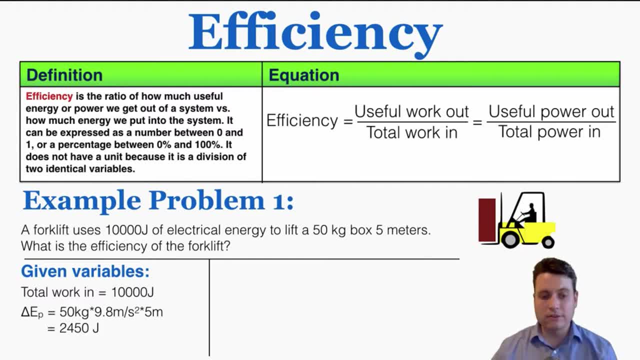 meters, which is 50 kilograms times 9.8, times 5,, just mass times, gravity times height, which is equal to 2,450 joules. So that's how much energy this forklift was able to turn into useful energy. 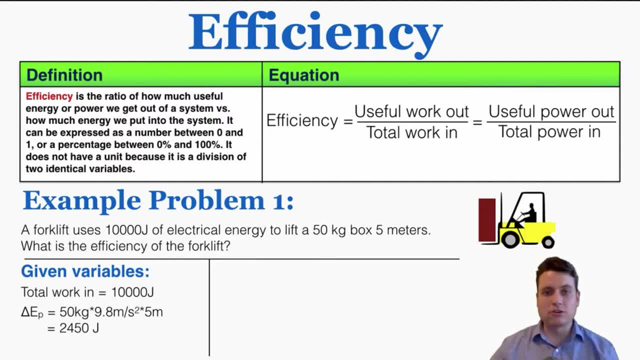 the good type of energy that we want in this case, which is gravitational potential energy. like a forklift is designed to give objects gravitational potential energy. So that means that the useful work out is also 2,450 joules, Because the efficiency is the useful work out over the total work in. that's going to be 2,450. 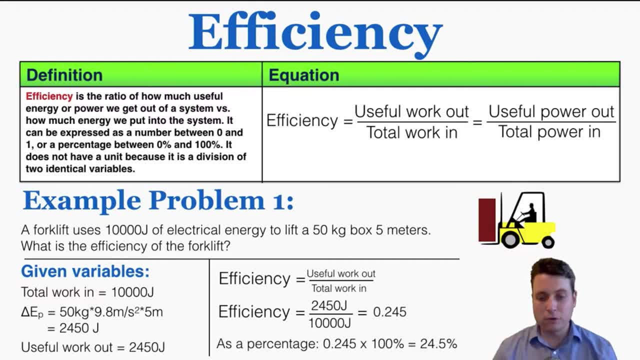 over 10,000, which is equal to 0.245, or 24.5%. To convert between a decimal and a percentage, you just multiply or divide by 100.. What this is saying is that this forklift is 24.5% efficient. 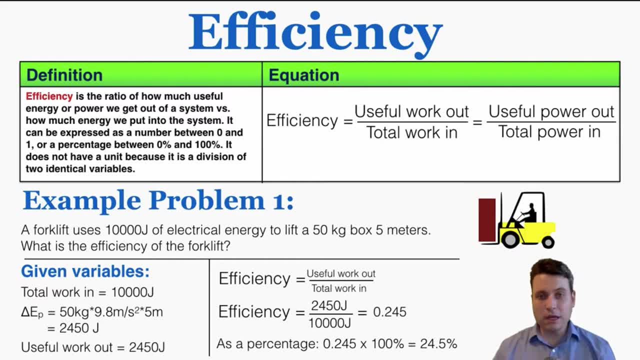 Whatever energy you put into the forklift as electrical energy, it's going to be able to use about 24.5% of that energy as useful gravitational potential energy. The rest of the energy is probably lost to heat, but it's going to be able to use about 24.5% of that energy as useful. 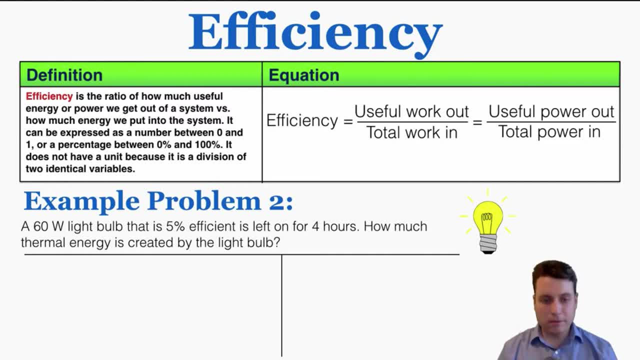 heat in the engine of the forklift. We can do another example problem: A 60-watt light bulb that is 5% efficient is left on for four hours. How much thermal energy is created by the light bulb? I'm going to start by rewriting the 5% as a decimal, because that's a little easier to do. 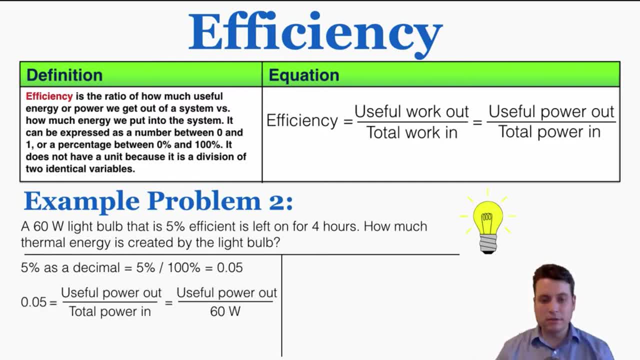 math with 5% is equal to 0.05 when written as a decimal. I know that 0.05 is equal to the efficiency, so that's equal to the useful power out over the total power in, and I know that the 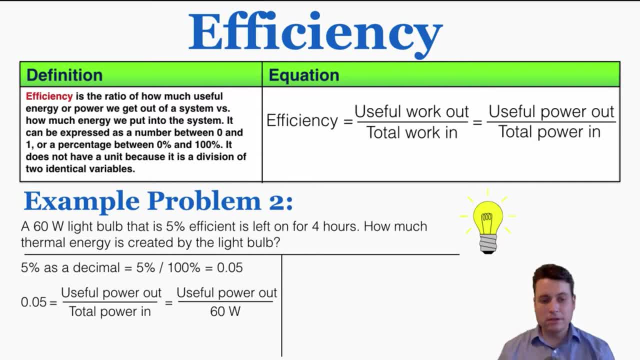 total power going into the system is 60, because it's a 60-watt light bulb, so that 0.05 is equal to the useful power that we're getting out of the light bulb divided by 60.. Using that setup, 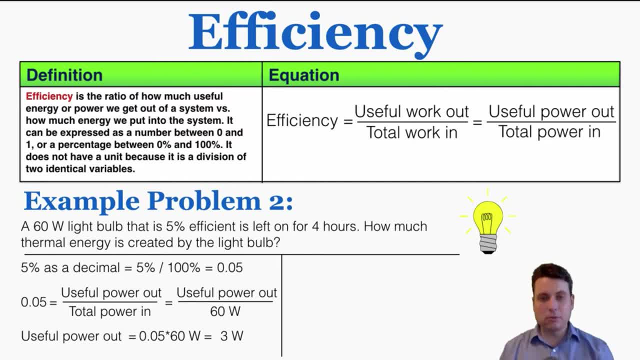 I can find the useful power that we're getting out of this light bulb. I can see that that's 0.05, remembering that efficiency doesn't have a unit times 60 watts, which is equal to 3 watts. But that's not what the question is asking about. It's asking about how much thermal energy. 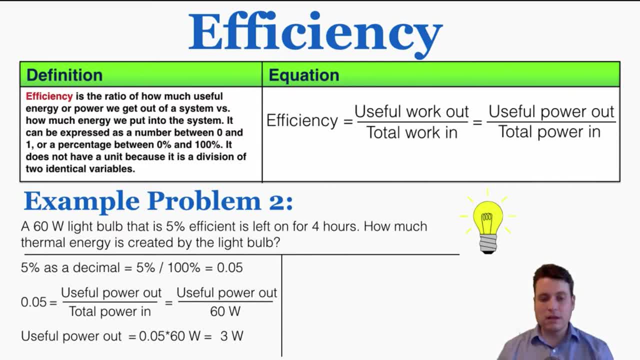 is created by the light bulb. If this light bulb really is 5% efficient, that means that when we put 60 watts in of electrical energy, we get 3 watts of radiant energy out, so the rest must be thermal energy. So that means that if we put 60 watts in of electrical energy, we get 3 watts of 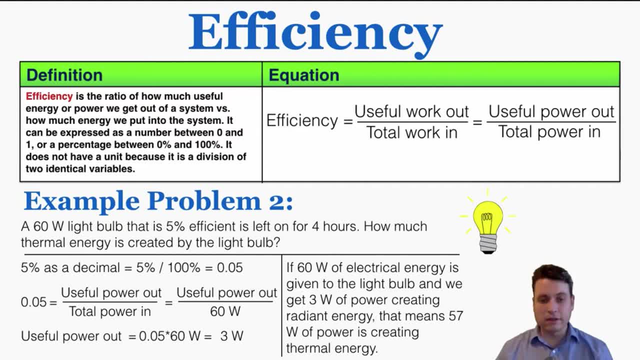 radiant energy. So that means that it's 57 watts of power. that's going into thermal energy specifically, and 57 watts of power means 57 joules of energy created every second. We can now solve the problem of how much thermal energy was created in four hours, because we know that. 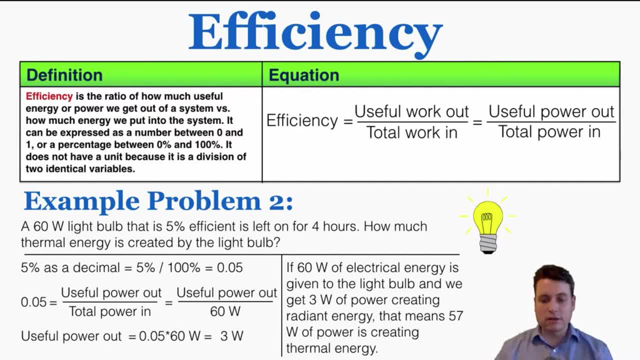 it's generating 57 watts of thermal power, which means that it's generating 57 joules per second of thermal energy. So that's the power that exists for thermal energy and this is the time, and we need that in seconds, because physics always measures time in seconds, Multiplying. 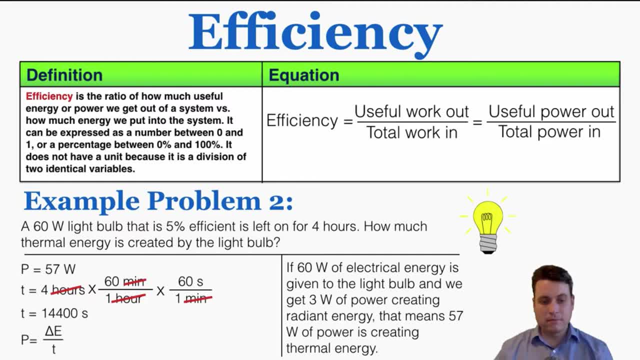 that out gets me 14,400 seconds, And power is the change in energy over time. so plugging that in 57 watts is equal to the change in energy over 14,400 seconds. Therefore the total thermal energy created by this 60-watt. 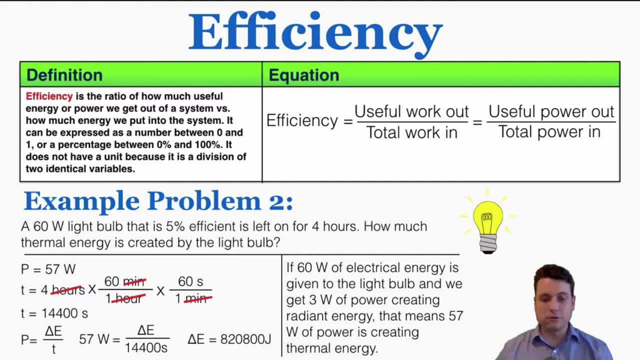 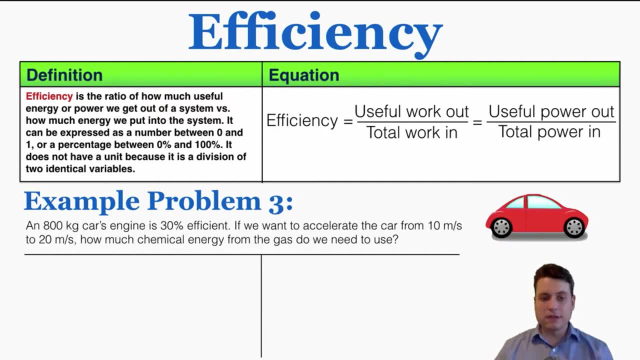 light bulb in four hours is 820,800 joules. It's pretty mind-blowing that a small household light bulb like that can create so much energy. Moving on to problem number three, an 800-kilogram car's engine is 30% efficient If we want to accelerate the car from 10 meters per second to 20 meters. 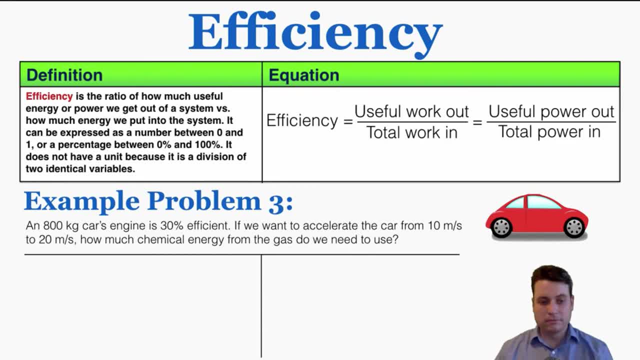 per second. how much chemical energy from the gas do we need to use? So I remember that work is equal to change in energy, and here I need to know the starting and final kinetic energy of the car, because we're changing the energy in some way and that additional 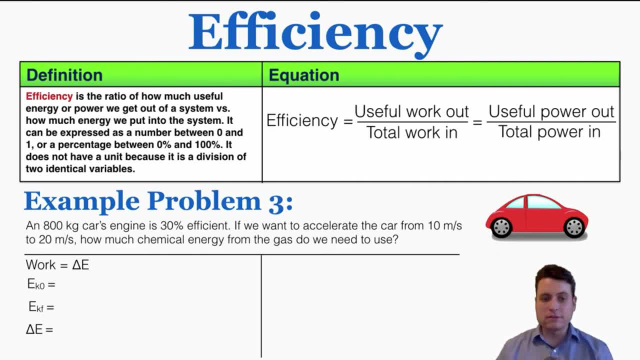 kinetic energy is the good, useful energy I'm trying to get out of this system. The starting kinetic energy of the car is one-half times its mass times its velocity squared, which is equal to 40,000 joules. The final kinetic energy is one-half times 800 times 20 squared, which is 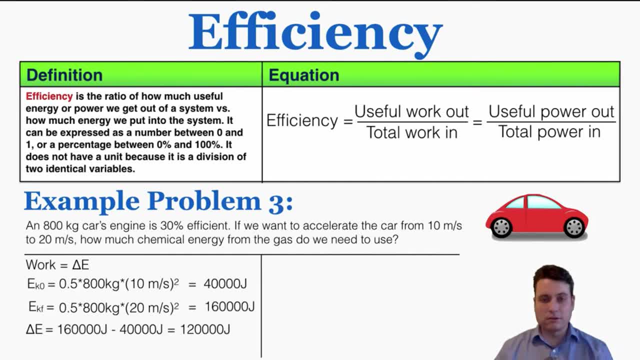 equal to 160,000 joules. so the change in energy is 120,000 joules. So that's how much useful energy is being added to the system. So the useful work out is 120,000 joules. And because the car is 30% efficient, I'm going to rewrite that as a decimal, which is 0.3.